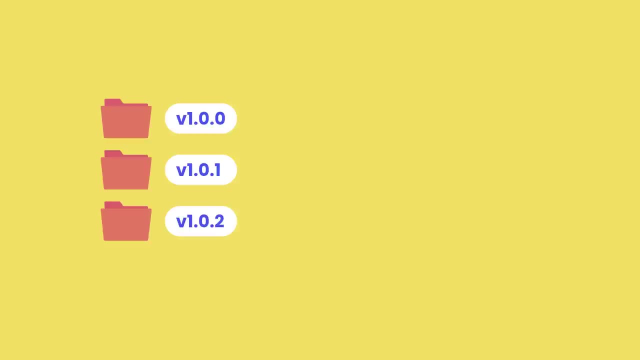 This is very slow and doesn't scale at all, especially if multiple people have to work on the same project. We would have to constantly toss around the latest code via email or some other mechanisms and then manually merge the changes. So, in a nutshell, with a version control system, we can track our project history and work together. Now version control systems fall into two categories: centralized and distributed. In a centralized system, all team members connect to a central server to 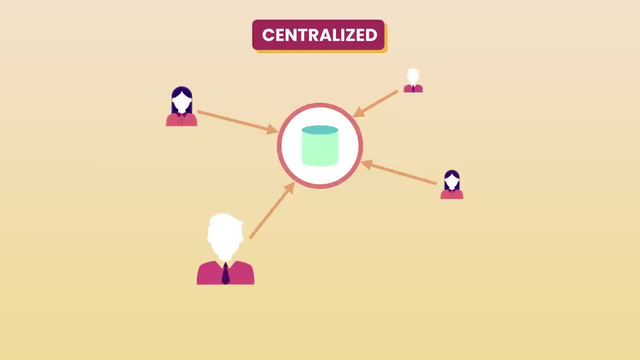 get the latest copy of the code and to share their changes with others. Subversion and Microsoft Team Foundation server are examples of centralized version control systems. The problem with the centralized architecture is the single point of failure. If the server goes offline, we cannot collaborate or save snapshots of our project, So we have to wait until the server comes back online. In distributed systems we don't have these problems. Every team member has a copy of the project with its history on their machine, So we can 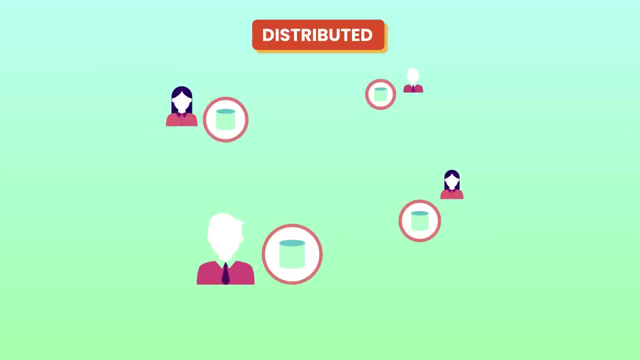 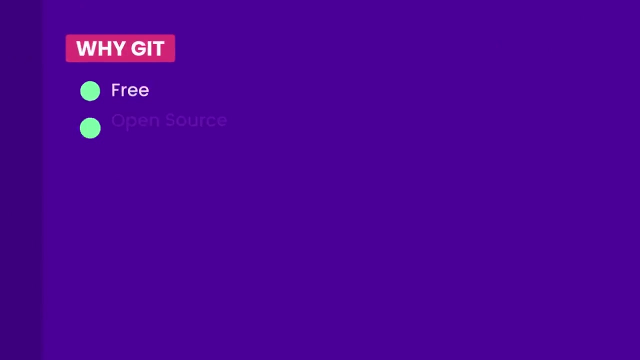 save snapshots of our project locally on our machine. If the central server is offline, we can synchronize our work directly with others. Git and Mercurial are examples of distributed version control systems. Out of all these, Git is the most popular version control system in the world because it's free, open source, super fast and scalable. Operations like branching and merging are slow and painful in other version control systems like Subversion or TFS, but they're very fast in Git. We'll talk about 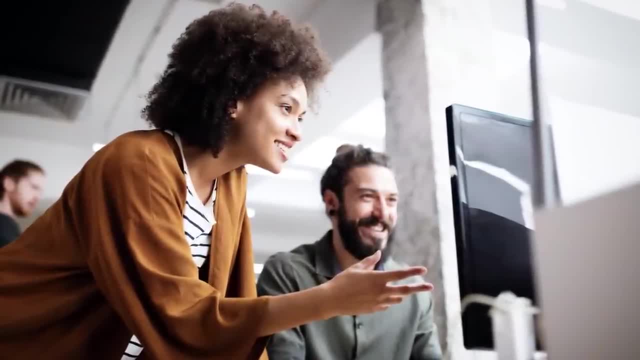 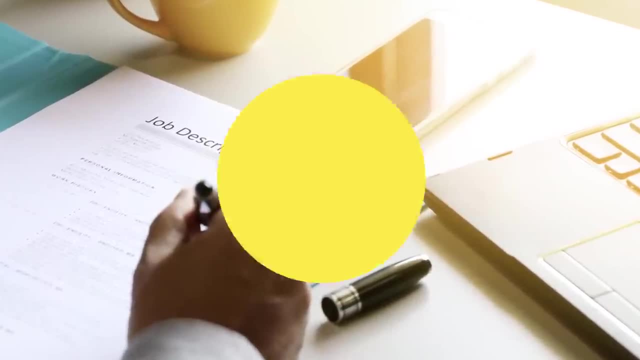 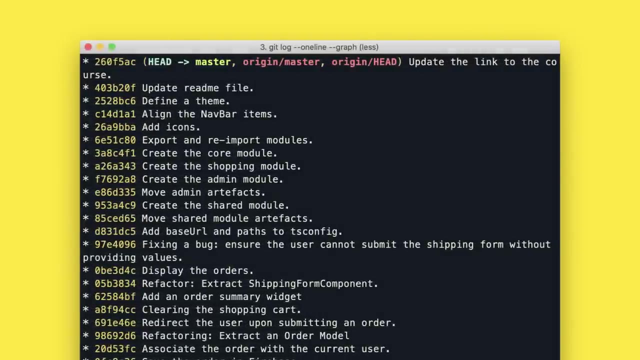 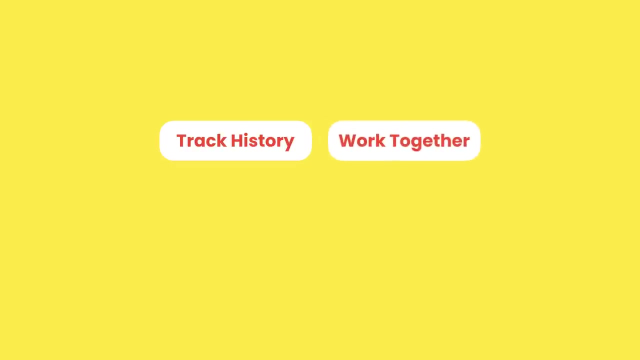 this later. So Git is almost everywhere. More than 90% of software projects in the world use Git. That's why almost every job description for a software developer mentions Git. So if you're looking for a job as a software developer, Git is one of the skills you must have on your resume. You should know it inside out. you should know how it works and how to use it to track your project history and collaborate with others effectively. If you want to learn Git, I have a one hour tutorial here on my channel. The link is below this video. If you enjoyed this video, 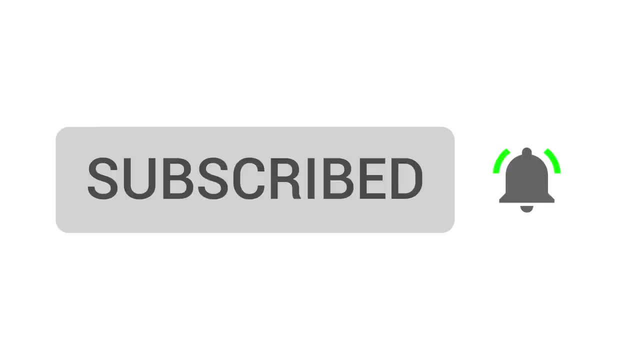 please give it a like and subscribe to my channel for more videos like this.